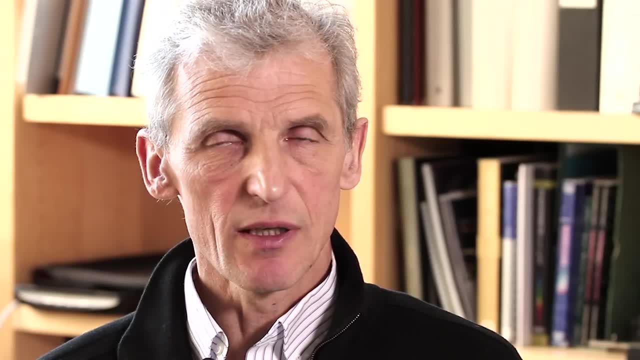 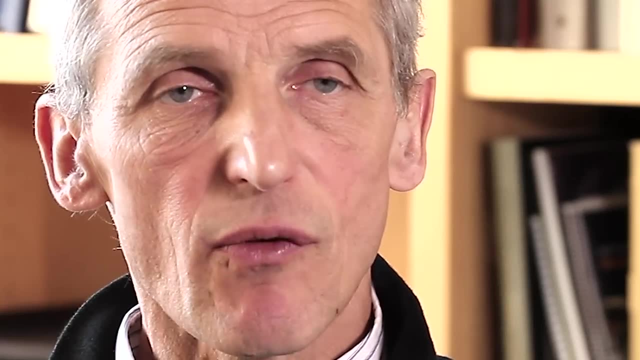 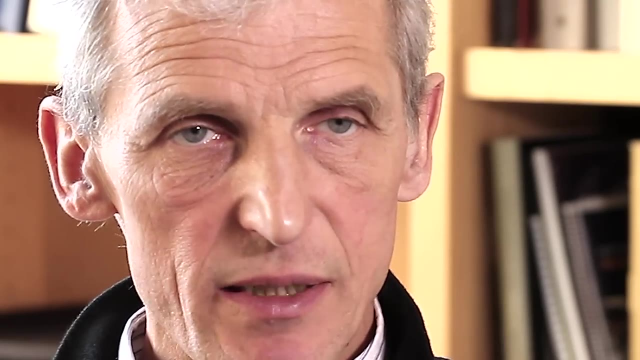 one big quantum wave. They consist of a macroscopic population of a quantum state. So Bose-Einstein condensation is a phase transition. when you cool down a gas of particles At higher temperature, you have random motion, and then at a very precise temperature you 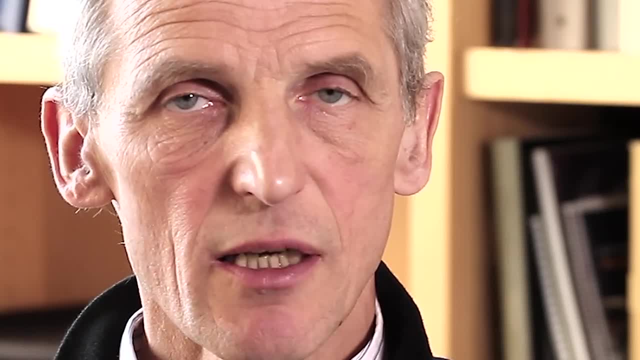 have a phase transition to this new form of matter called Bose-Einstein condensation. Bose-Einstein condensation is a new form of process. It is performed by changing the energy at higher temperatures, by wave cycles. For example, if you are earthen wool, you 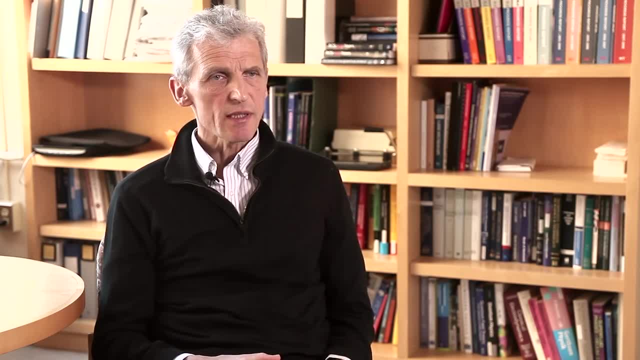 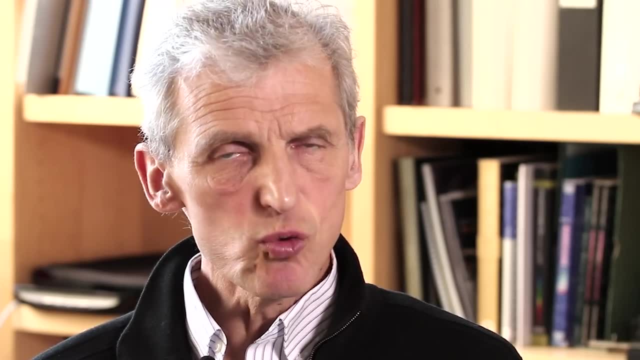 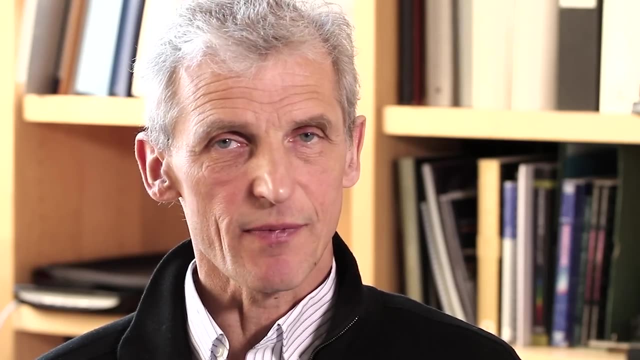 It's the consequence of quantum statistics, it's the consequence of the indistinguishability of particles. and in physics we have two kinds of particles: bosons and fermions. and Bose-Einstein condensation only occurs for bosons. Why do we have only two kinds of particles, bosons and fermions? Well, in physics we classify bosons and fermions whether they have integer or half-integer spin. But for laypeople I can give an easier definition, and that is that at low energies in the world around us all particles consist, all composite particles like atoms and molecules consist. 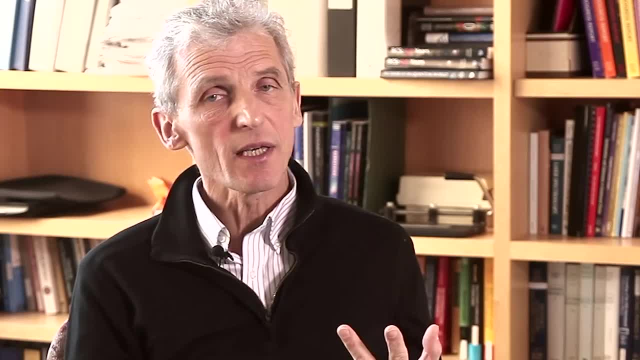 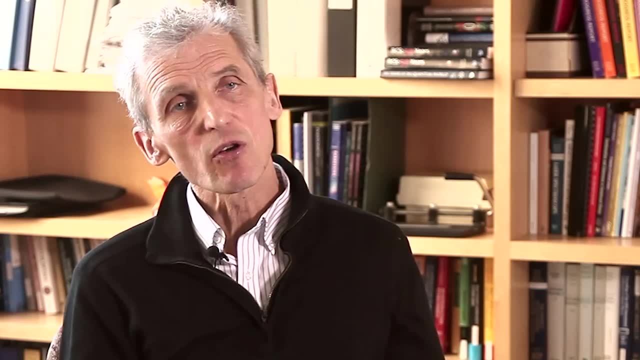 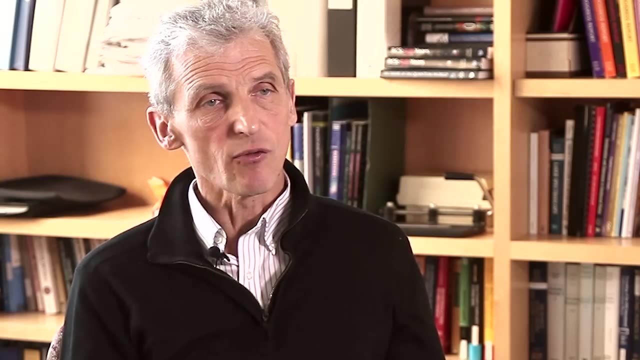 of protons, neutrons and electrons. And now we can classify all those particles whether there is an odd or even number of constituents. If the number of constituents is even, we call this particle a boson. If the constituent is odd, we call it a fermion. 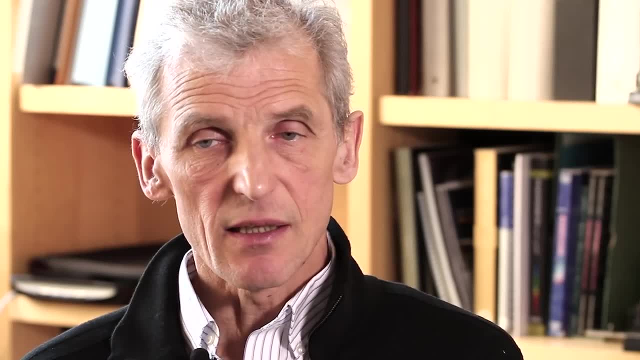 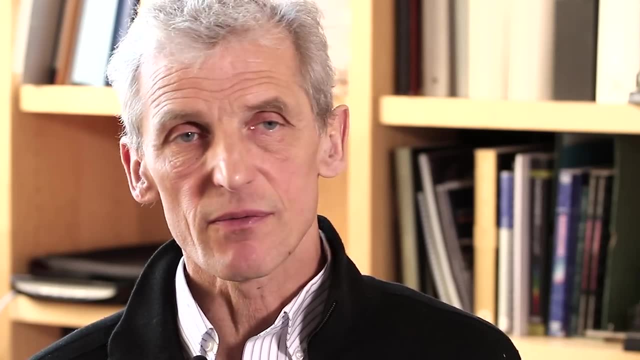 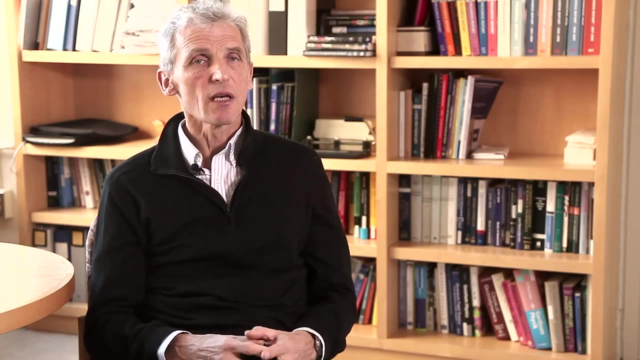 So only bosonic particles can undergo Bose-Einstein condensation. but many atoms in nature are bosons. So if you take a gas of bosons- and the first experiments were done with alkali atoms, sodium and rubidium- and we cool it down to low temperature, 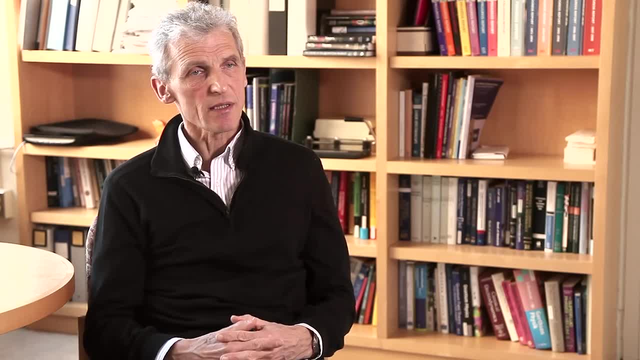 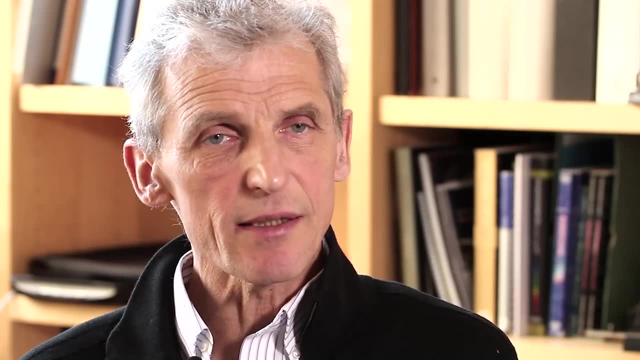 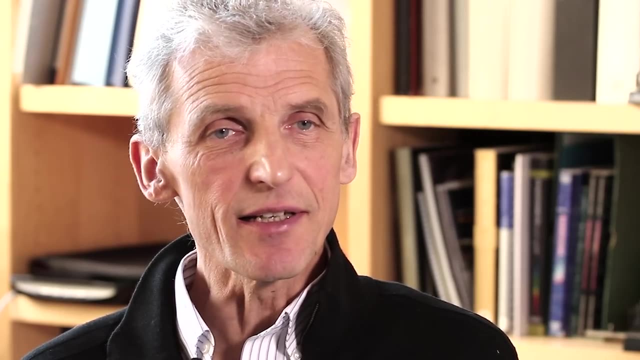 Then we can observe this spectacular phase transition into Bose-Einstein condensation. The fact that Bose-Einstein condensation was predicted in 1925 and observed in the laboratory only in 1995, 70 years later- indicates that there were certain challenges in realizing. 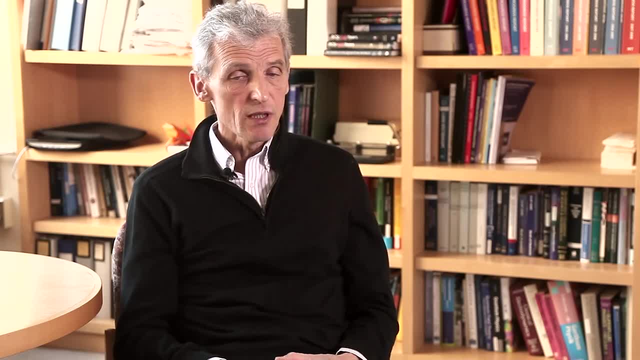 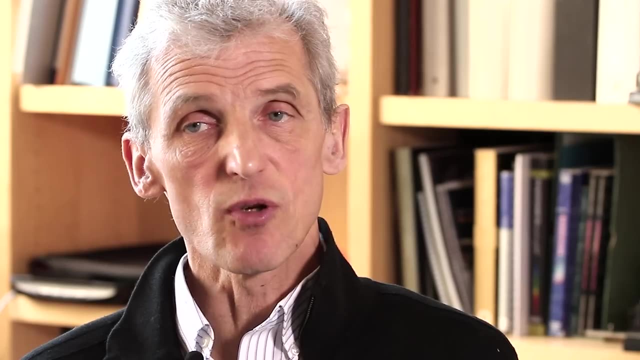 Bose-Einstein condensation. We know now that Bose-Einstein condensation can only be achieved when you cool gases down to nano-Kelvin temperature. Nano-Kelvin is a billionth of a degree Kelvin, so you have to go very, very close to absolute. zero. Just to put it in context, nano-Kelvin temperature is more than a million times colder than interstellar space. So it was only in the 80s, with laser cooling, and the 90s, with the addition of evaporative cooling, that we had the technology, the cooling techniques, to take a gas and cool it down. 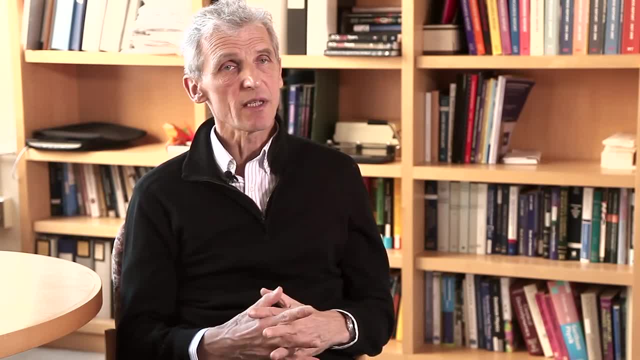 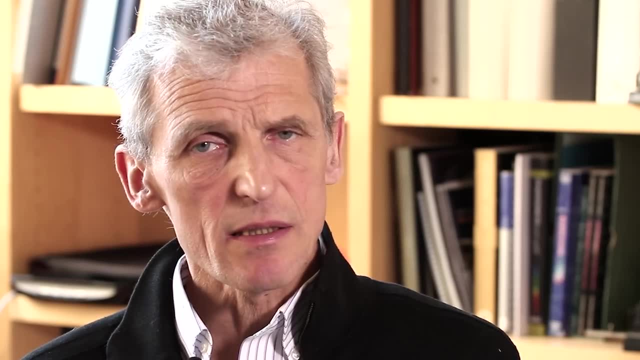 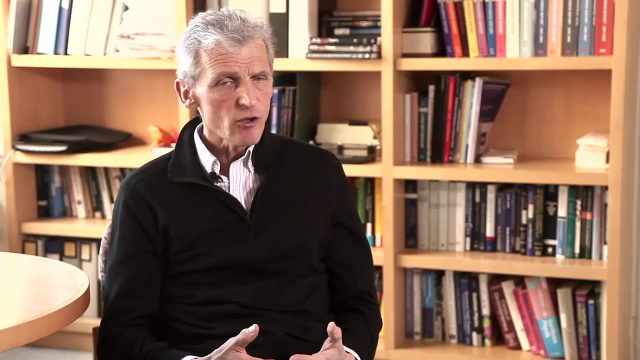 Now you take a gas of atoms and cool it to nano-Kelvin temperatures where Bose-Einstein condensation can be observed In thermal equilibrium gases are described by statistics, by thermodynamics, by quantum statistics. In quantum statistics we have a mathematical expression which tells us how many particles. 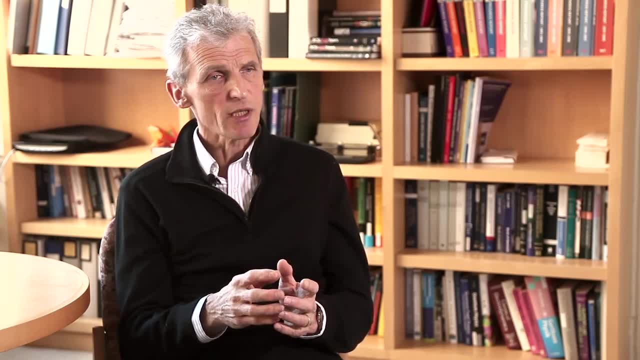 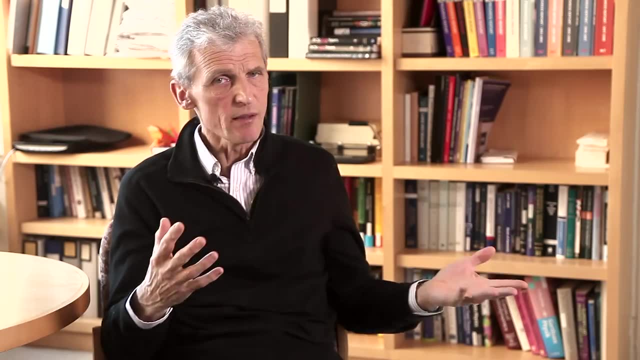 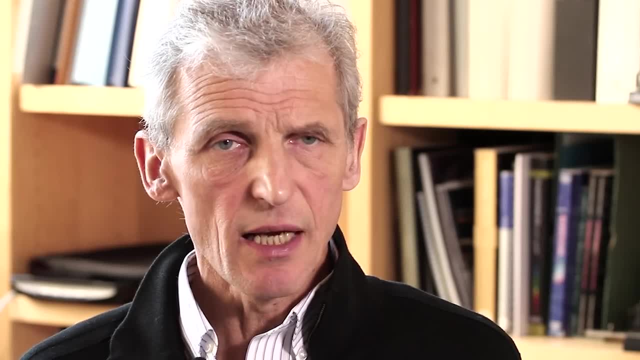 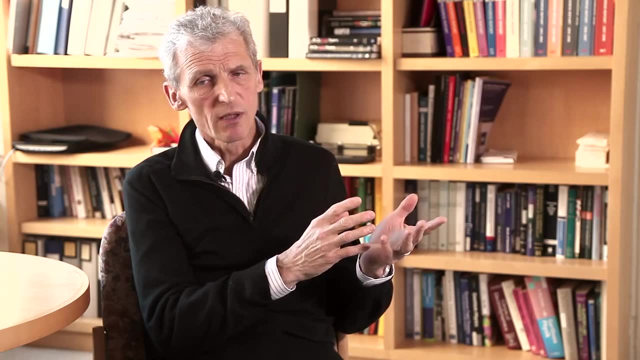 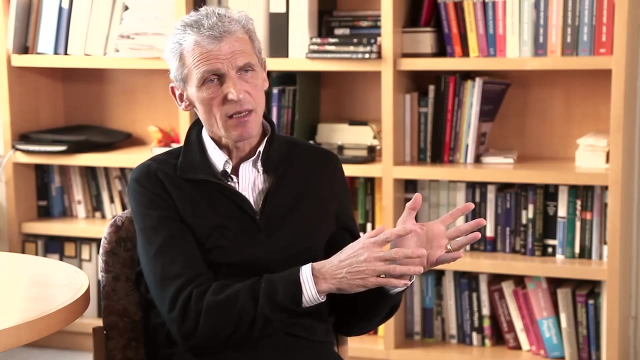 emotional states. In a Bose-Einstein condensate, we have a macroscopic fraction of the particles in a single quantum state And this transition from occupying many states to predominantly occupying a single quantum state. this is what suddenly happens at the phase transition of Bose-Einstein. 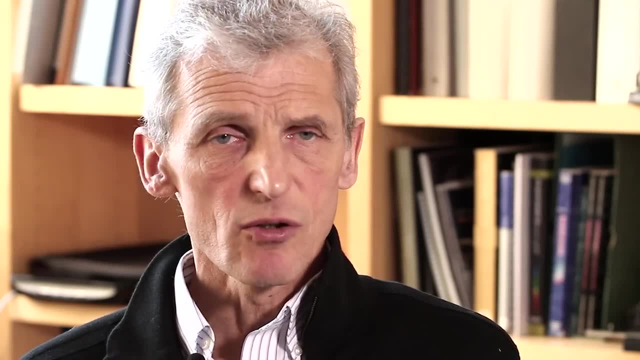 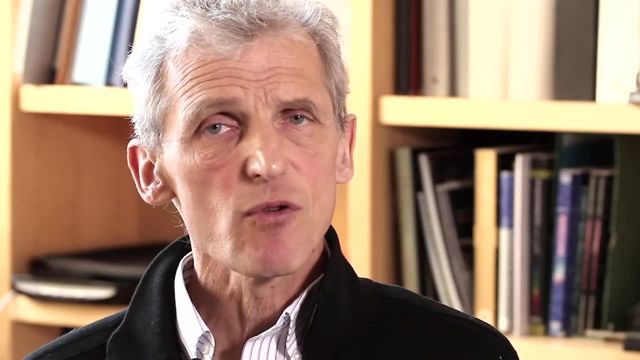 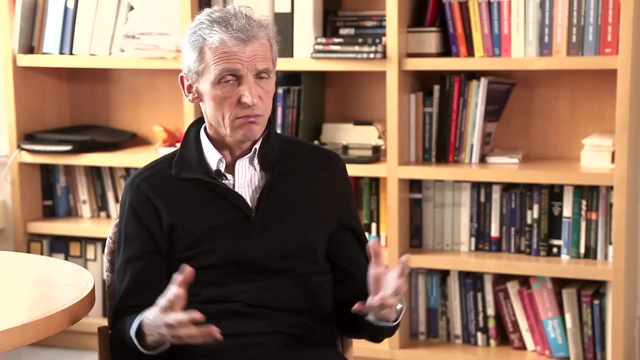 condensation. I've just mentioned the challenge to pursue. Bose-Einstein condensation was the accomplishment of very, very low temperature. However, there was an additional challenge. You can call it a conceptual challenge. If you cool down, you know any form of matter to very low temperature, what happens? Well, all. 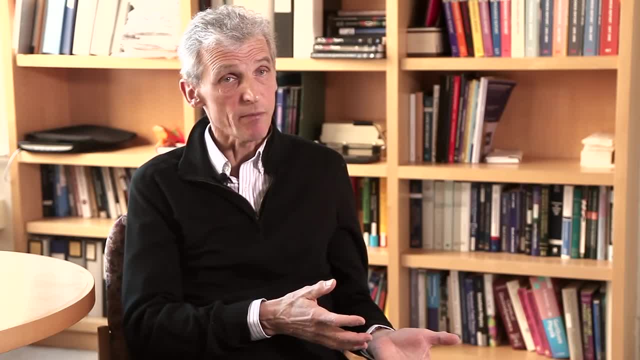 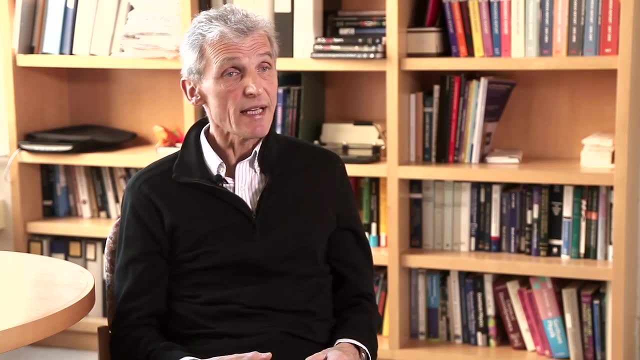 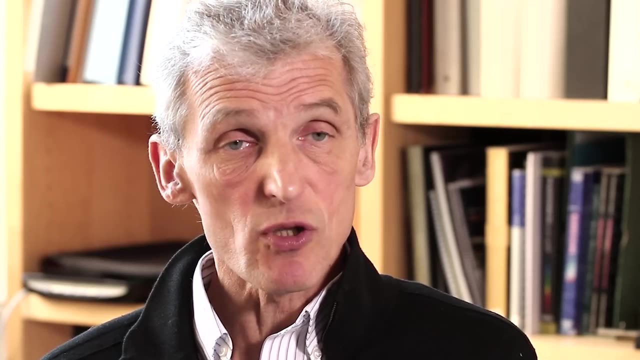 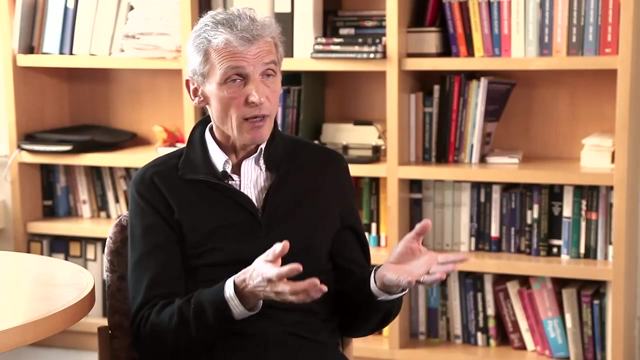 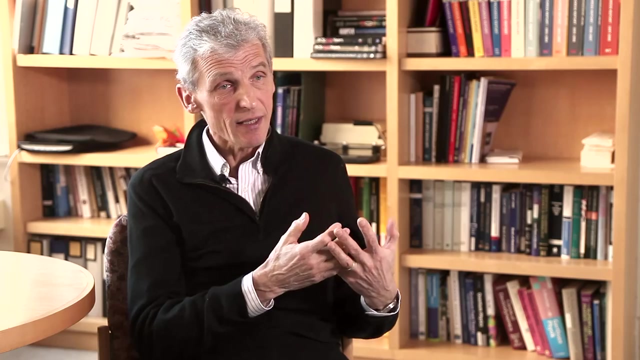 matter liquefies and solidifies at low temperature. But Bose-Einstein condensation is very, very low temperature And that's why we have to think about it, Because if you cool down you know any form of matter to very, very low temperature. But Bose-Einstein condensation is about a special phase, a special property of a gas of particles. So from that you would conclude: Bose-Einstein condensation, how it was described by Einstein in an idealized way, cannot be realized in nature. because before atomic gases would form a Bose-Einstein condensate, they would first freeze, liquefy and solidify. And there are famous physicists who have written a lot of 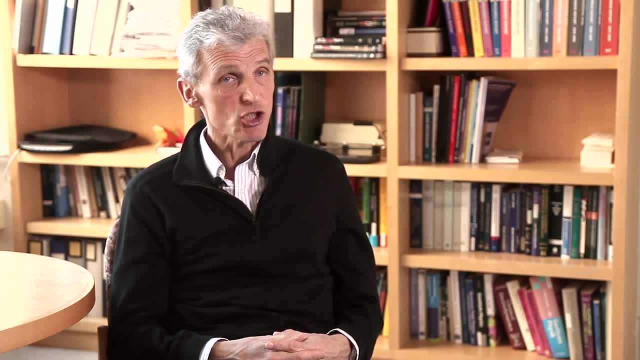 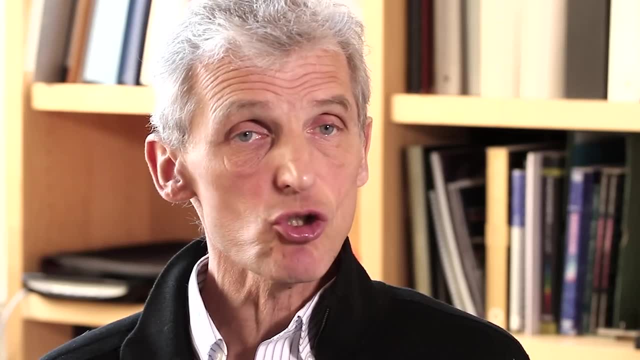 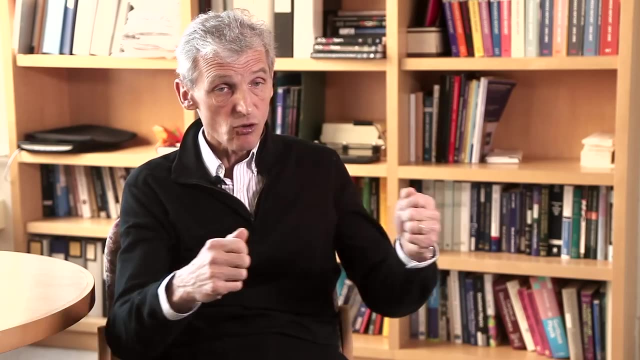 that Bose-Einstein condensation will never be achieved. However, in the 70s people realized that Bose-Einstein condensation should be possible in a metastable form. When you have a very dilute gas, particles can collide, and still through collisions. 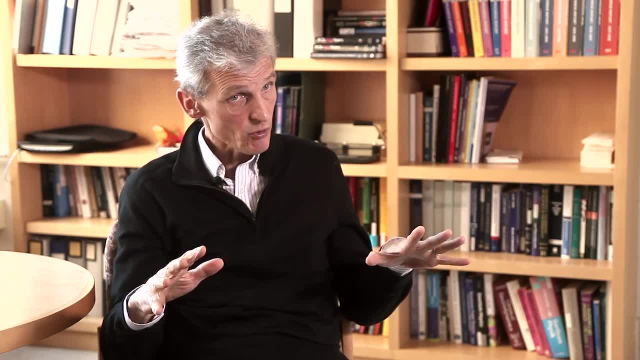 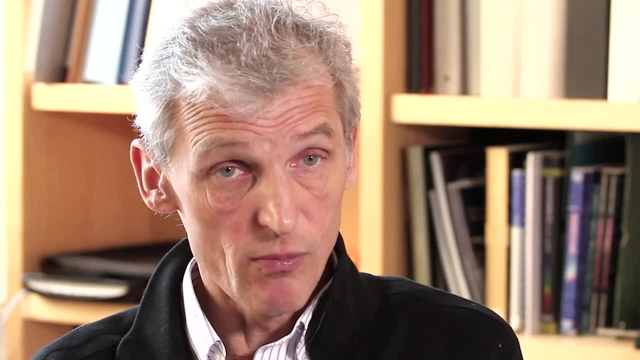 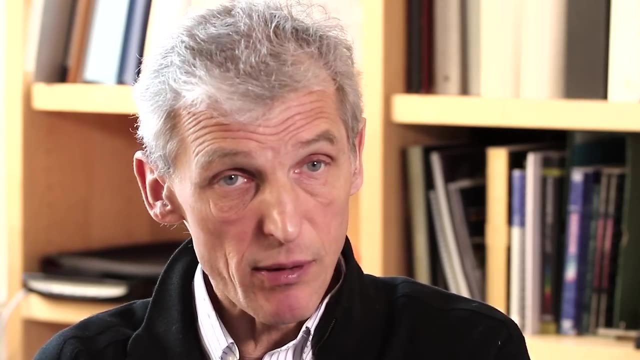 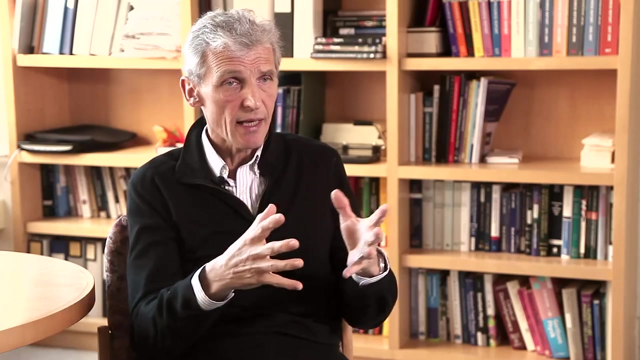 establish an equilibrium velocity distribution. However, the step to form a cluster, form molecules, form liquid droplets and form a solid requires not only two particles to come together, but at least three. Otherwise you cannot. in order to have formation of some higher aggregate and to conserve momentum and energy, you need more than two particles colliding. 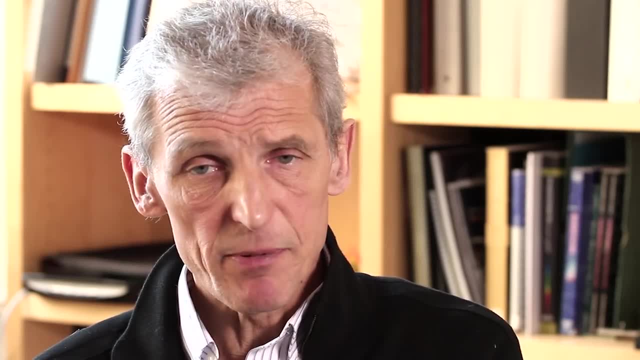 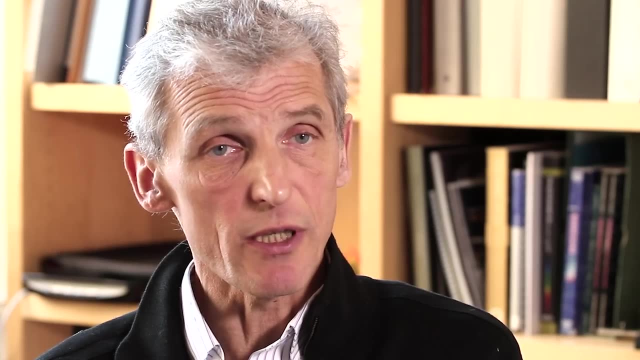 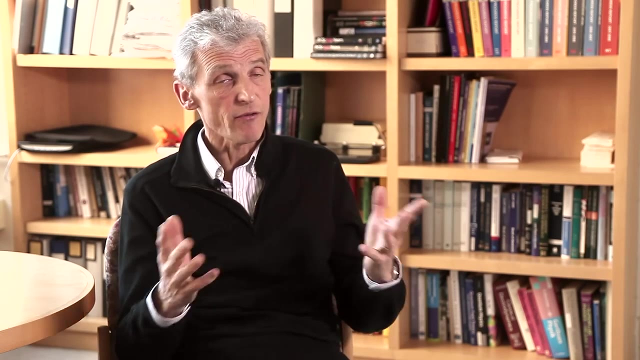 So, in other words, the step towards aggregating matter to liquids and solids. this requires a at least three body collisions, and if you go to a very, very dilute gas, you have lots of two-body collisions but you have virtually no three body collisions. 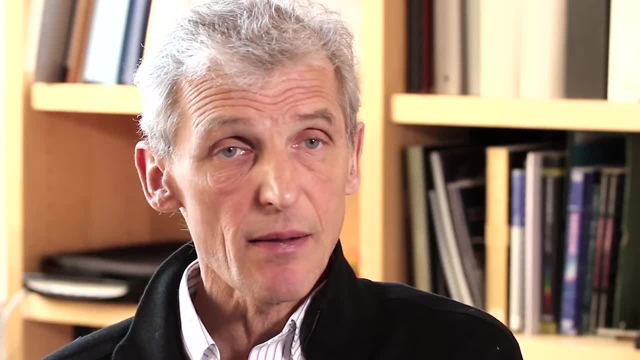 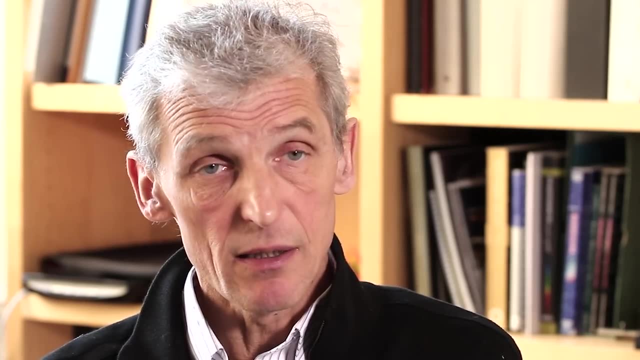 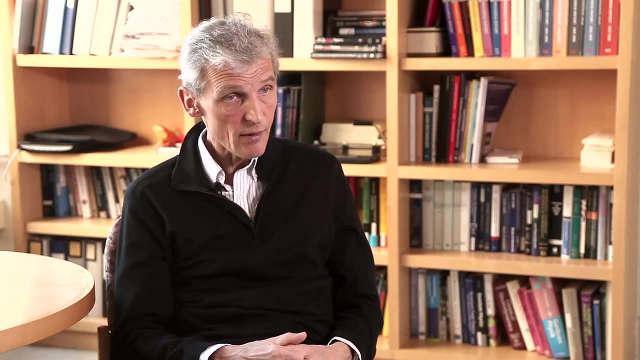 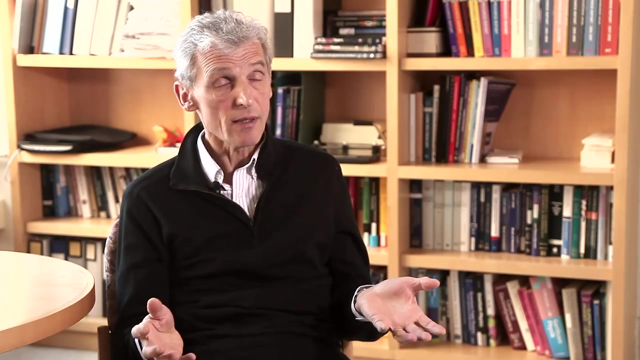 So, in other words, people realized that at very low density you may still have equilibrium of the gas, but the pathway to liquification and solidification are dynamically suppressed. In other words, we can study a gas gas, although the gas is much, much, much colder than the temperature for solidification. 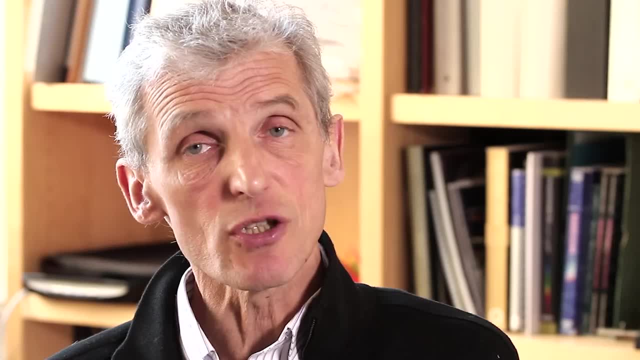 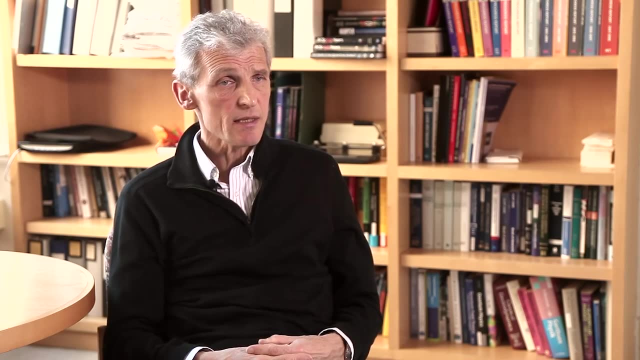 So we are in a metastable phase and this is the regime in which all the experiments of Bose-Einstein condensation are carried out. So in the 70s people realized that Bose-Einstein condensation should be possible, but the only. 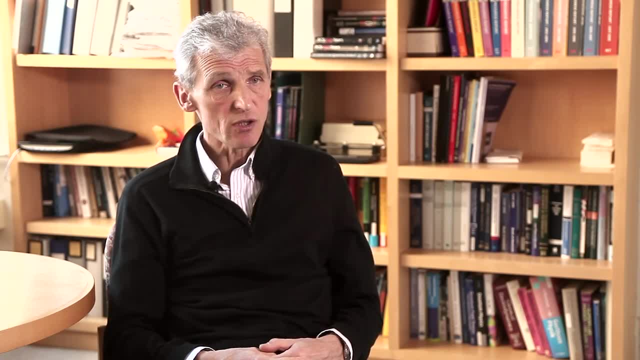 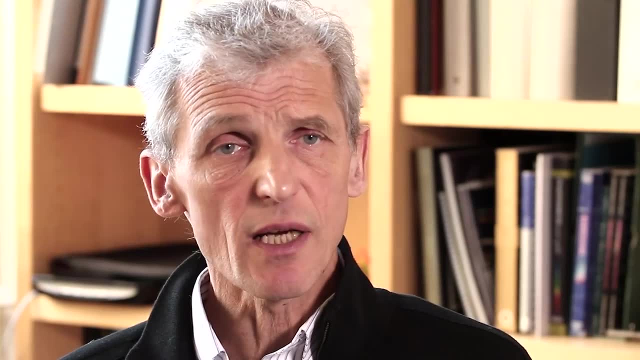 candidate for Bose-Einstein condensation was atomic hydrogen. So in the 70s, people started to pursue atomic hydrogen and eventually, in 1997 or 1998, Bose-Einstein condensation of hydrogen was achieved after 20 years of research. 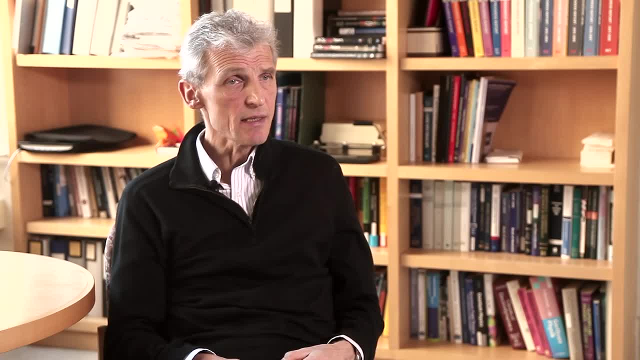 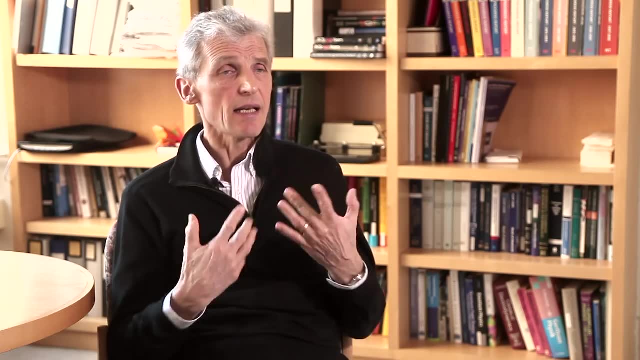 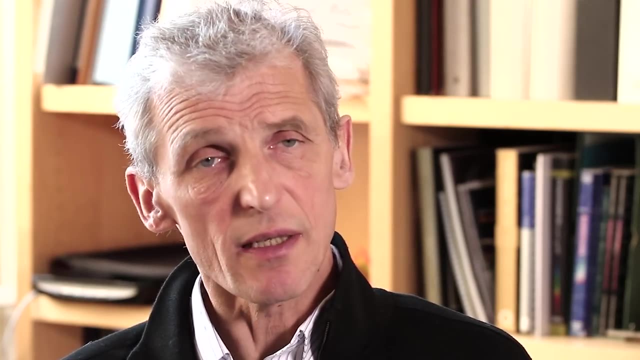 However, in the mid and late 80s laser cooling of atoms had been invented and now there were other candidates, laser-cooled atoms, for the pursuit of Bose-Einstein condensation, And it was a combination of laser cooling- There was cooling and evaporative cooling, which led to the big breakthrough in 1995.. 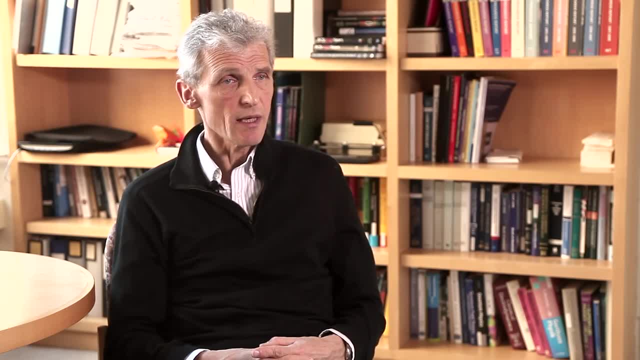 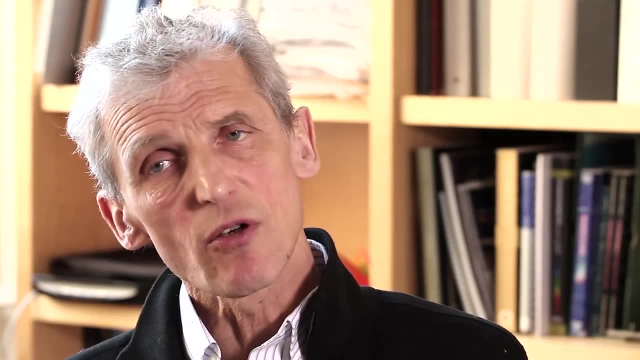 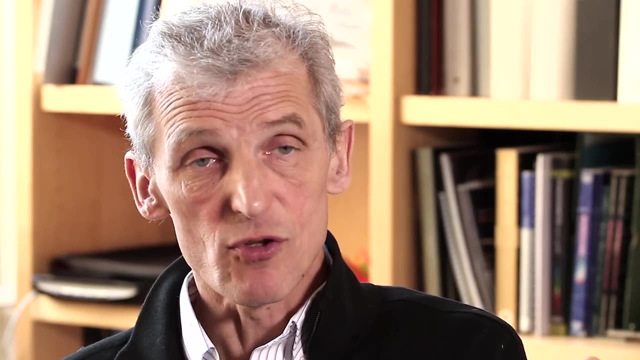 And today the whole field is completely dominated by the species which are first laser-cooled and then evaporatively cooled. When people pursued laser cooling of atoms, they wanted to go to lower and lower temperature, And what was regarded as the ultimate goal was to cool a gas down to Bose-Einstein condensation. Because the Bose-Einstein condensate is a gas. It's the ultimate low-temperature phase of a weakly-interacting gas. So if you ask, at the lowest temperature close to absolute zero, what happens to a gas of bosons? well, it forms a Bose-Einstein condensate. 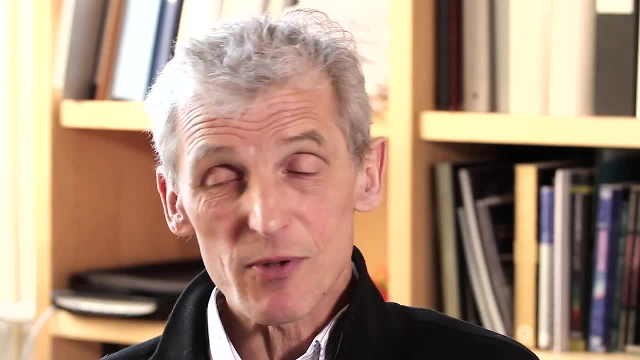 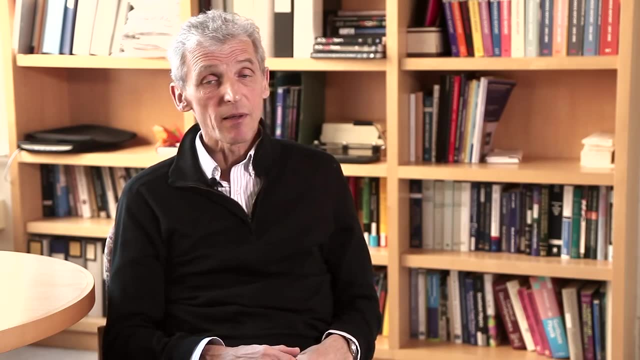 So when we realized Bose-Einstein condensation in 1995, we thought this would be pretty cool and we realized that we could now study superfluidity and some other aspects of cold matter. But what I hadn't fully realized is that the accomplishment of nano-cannabinoids, which 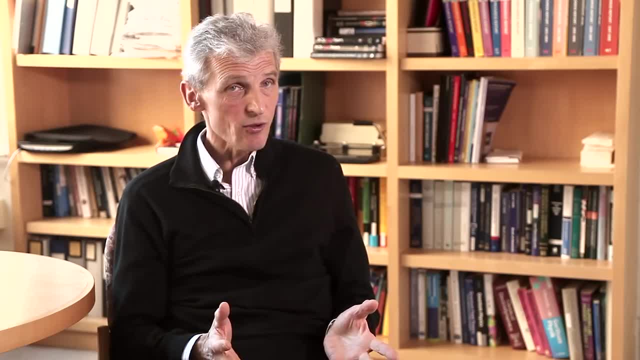 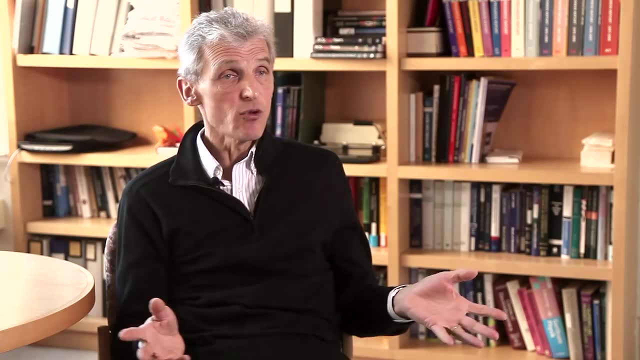 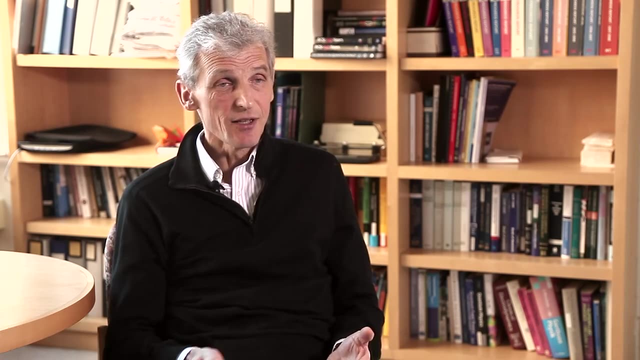 have a low Kelvin temperature was not just good for Bose-Einstein condensation. It opened up a host of new scientific directions. It's a little bit like if you invent a refrigerator and the first thing you cool down in your refrigerator is you cool atoms to Bose-Einstein condensate. 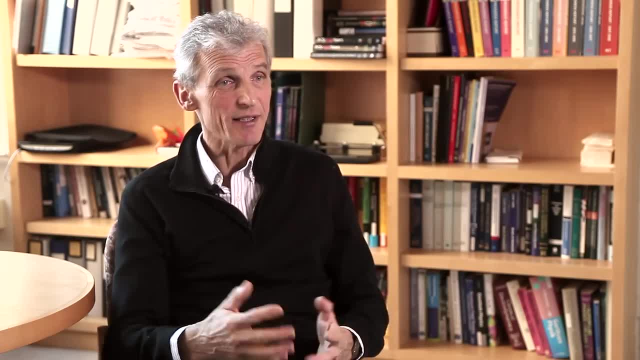 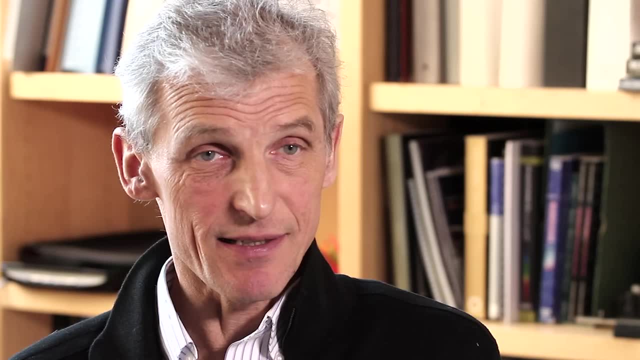 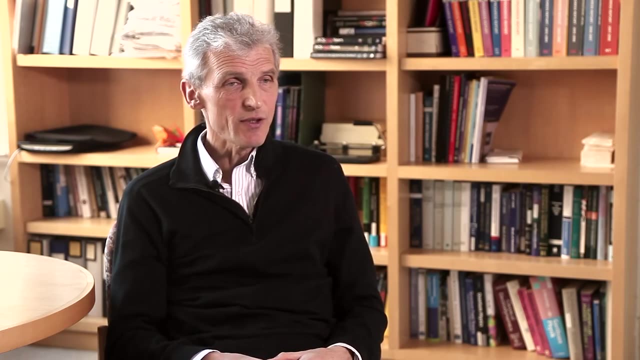 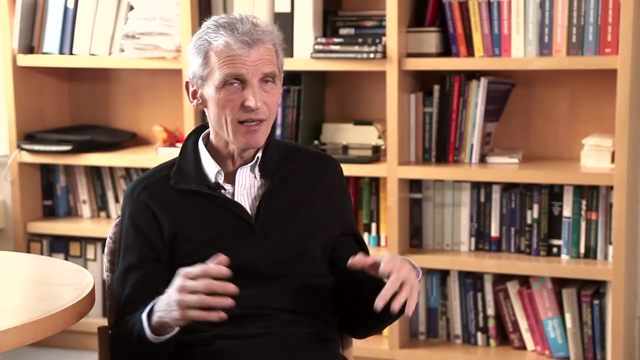 You can now put all sorts of different forms of matter into your refrigerator, and the number of possibilities- what you can study- is practically endless. Now, more than 15 years after the discovery of Bose-Einstein condensation, the field is still brimming with excitement, and there are lots of new directions and new discoveries. 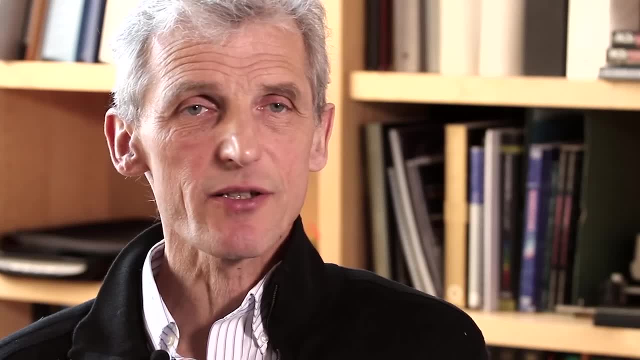 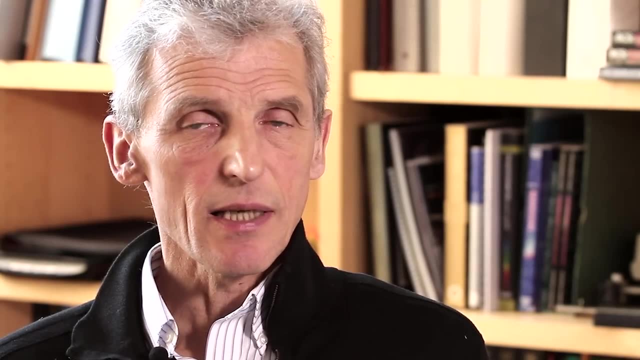 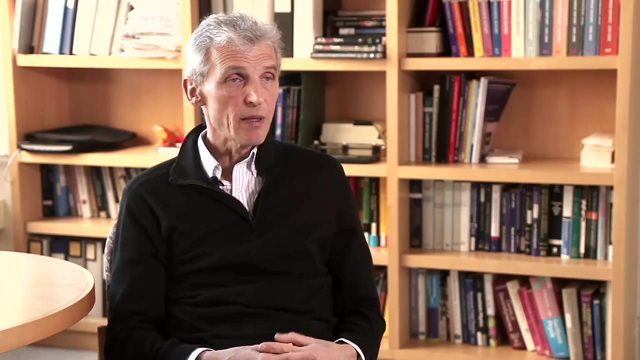 and breakthroughs every year. What came after Bose-Einstein condensation? Well, people studied the properties of the Bose-Einstein condensate, but then they extended the cooling techniques to Fermi gases. So superfluidity- Superfluidity of fermions- was studied. 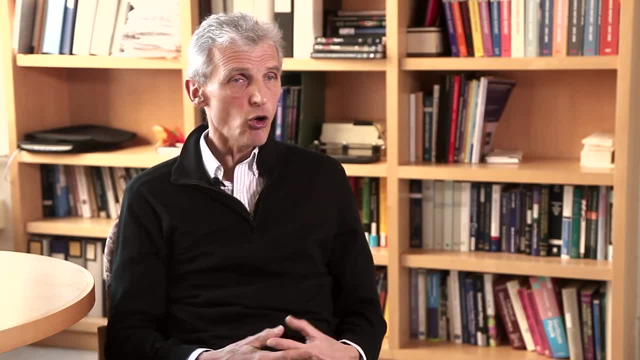 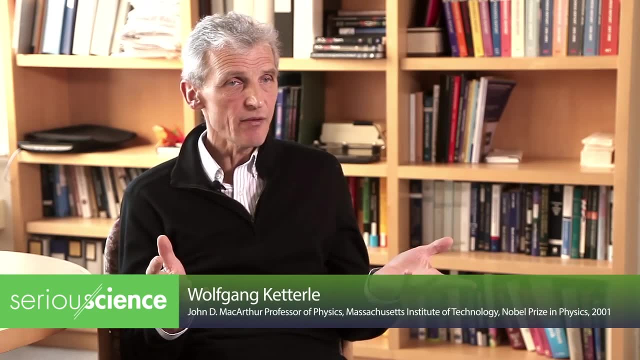 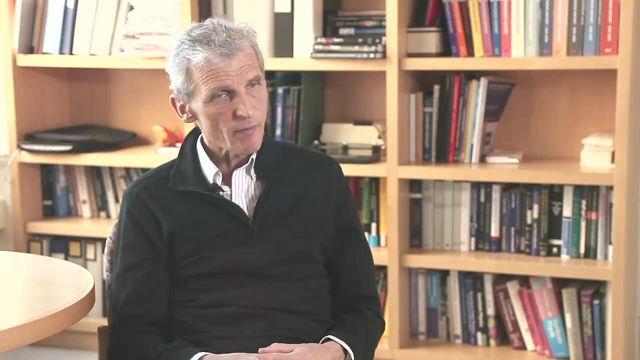 People used additional laser beams created what we call optical lattices, periodic arrays of atoms like in a crystal. We observed insulating behavior and now one of the hot topics is quantum magnetism: study magnetic properties of ultracold matter. What are you looking for?